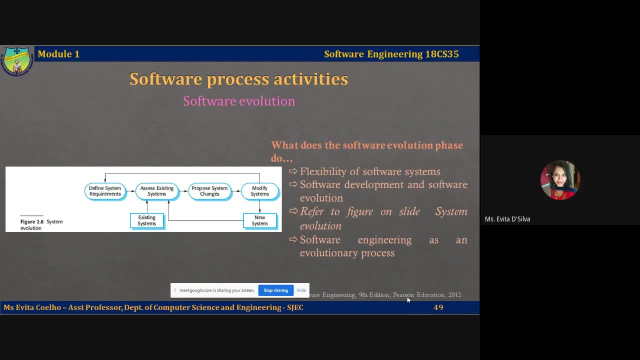 there has always been a split between the process of software development and the process of software evolution or maintenance. People think of software development as a creative activity in which a software system is developed from the initial concept through to a working system. However, people also think software maintenance as dull and uninteresting and maybe not the task of an 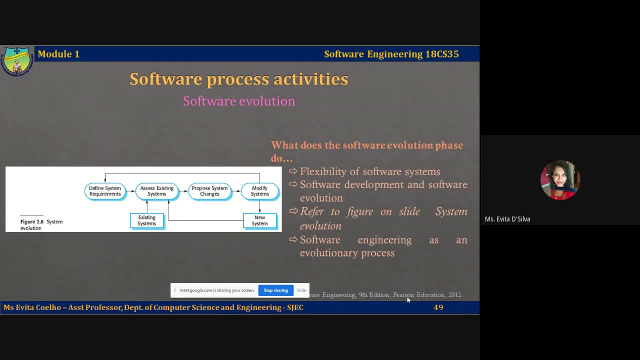 engineer, Although the costs of maintenance are often several times higher than the initial development costs, maintenance processes are sometimes considered to be less challenging than the original software development. This distinction between development and maintenance is increasingly irrelevant. Hardly any software systems are completely new systems, and it makes 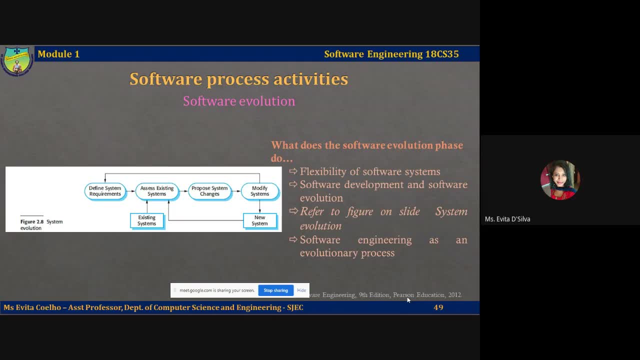 much more sense to see development and maintenance as a continuum, given the fact that most of the times we try to assess and reuse existing software systems Rather than two separate processes. it is now more realistic to think of software engineering as an evolutionary process, where software is continually changed over its lifetime. in response, 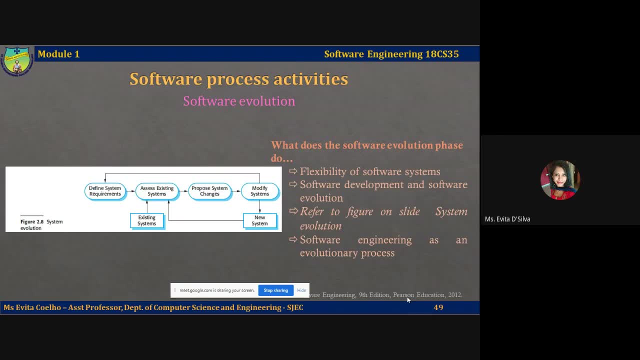 to changing requirements and customer needs. Let's take a look at the diagram depicted on the slide. This figure shows system evolution. If we look at the first phase of system evolution, it talks about defining system requirements. We may get the system requirements from the customer in the form of a system requirement or requirement specification. 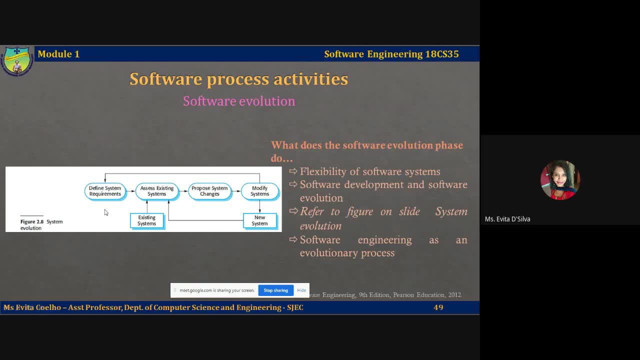 We may add our own system specification depicting the requirements of the system that is going to be developed based on customer requirements. Once we have the system requirement in place, we are going to go to the next phase Here, rather than developing a software system from scratch. 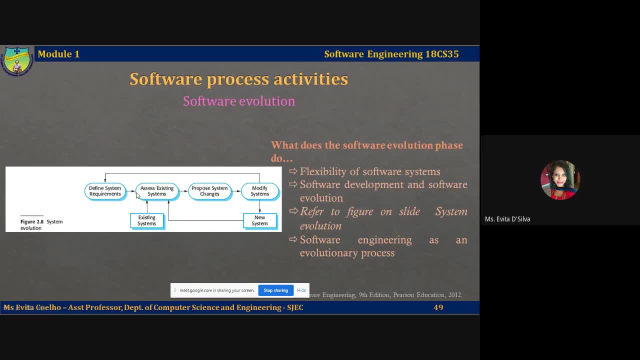 we are going to assess the existing software systems which provide the similar functionality. So you have a database of existing systems and you are going to assess these systems and see if there exists a software system that closely matches to your requirements. If so, you are going to take that up and propose a few changes to that system in order to make that.